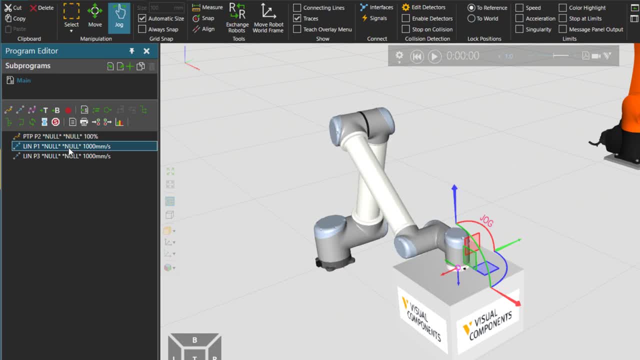 So I'm going to approach this point: go to the box, grab it and go up, So, and then to grab it, I need a signal and then a set binary output statement. So these are the main statements that you can use inside a robot program, And I'm trying to show you the most common ones. 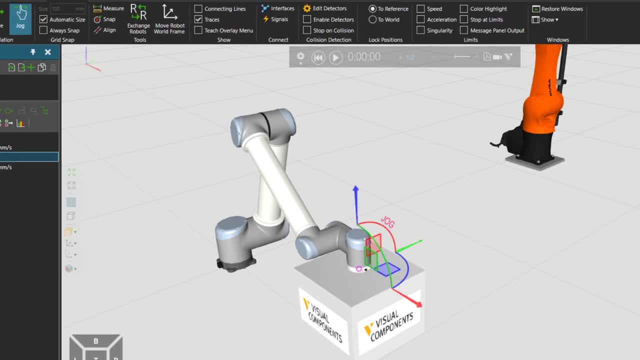 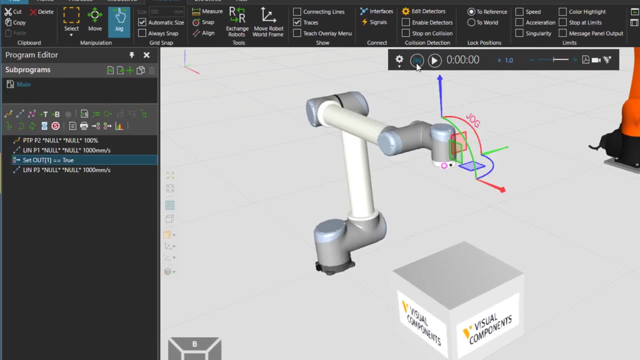 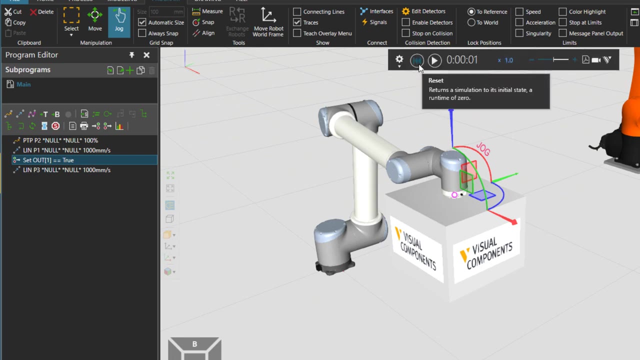 right now. So to grab the box, I need to set output. So I'm going to set the output port one to true, meaning that I will grab the box when the signal is set. So the box is now in air. And then, in case you want to set a different, 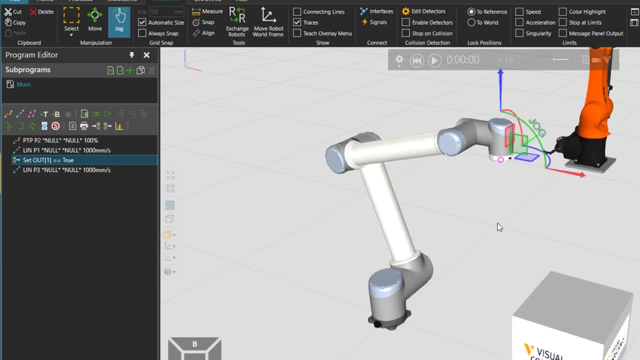 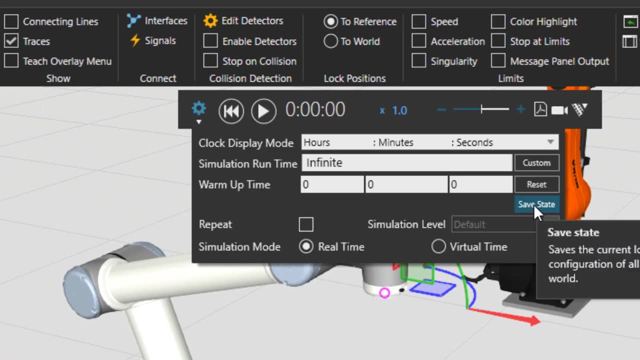 initial position. for example, let's say we want the robot always to start from here. you can set it and then go to the gear button. There is also a save state here And then, as you can see, the robot is now in air. That means that that position is saved for. 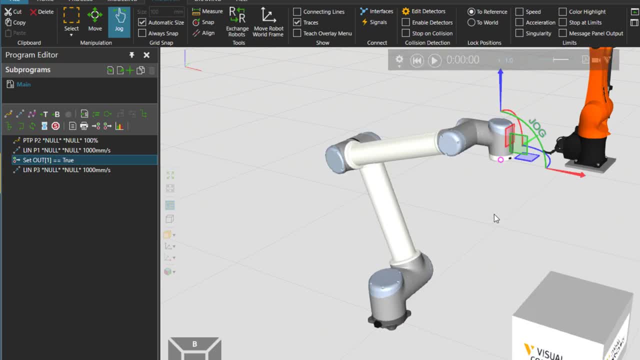 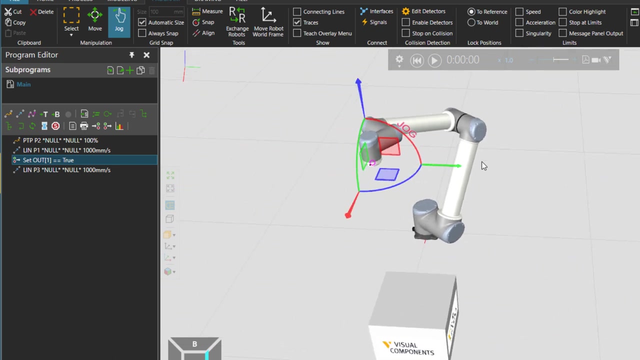 the robot. If I press reset, you see, it goes to that initial state I just set. The other way is to just set a specific state and then press play. That also saves the robot. joint values in the initial state. So you see, now this new one is chosen. 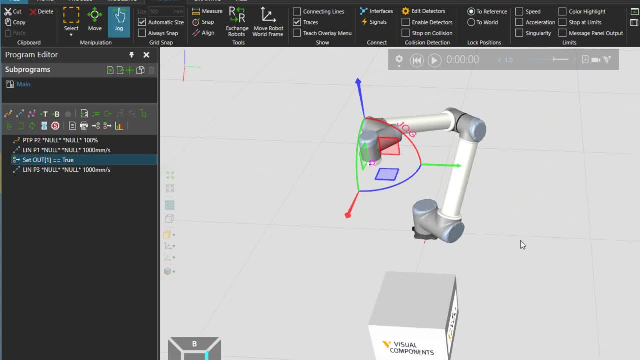 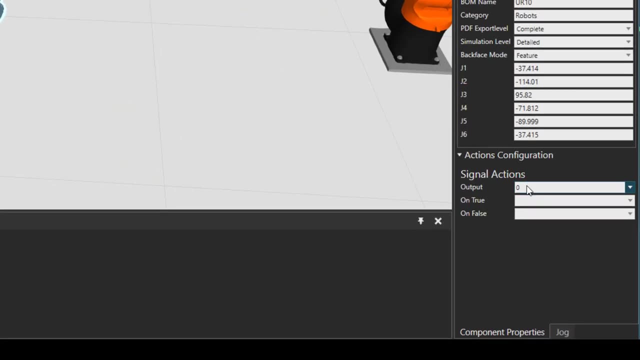 And how did I know that signal output one is for grabbing the box. Well, click on the robot, Go to signal robot property panel and then actions configuration and then choose the output number one and you see the details over here. So this is for grasping and releasing this signal. 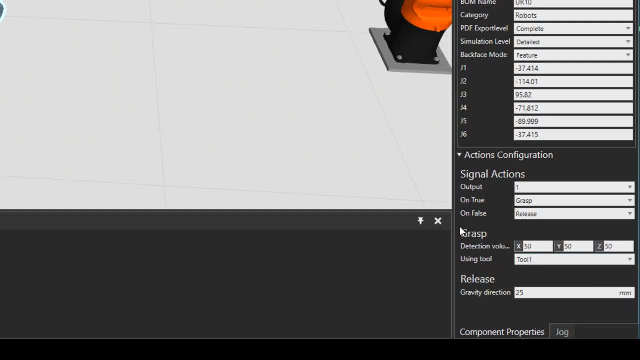 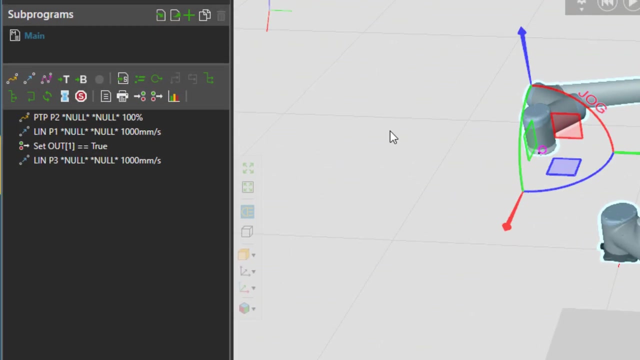 And then the tool that we use for this is also mentioned here. As a rule of thumb, the first 100 signals in visual components are booked for the robot programming purposes, And if you want to set on your own signals, you should start after 100.. You can see what each signal does over here. 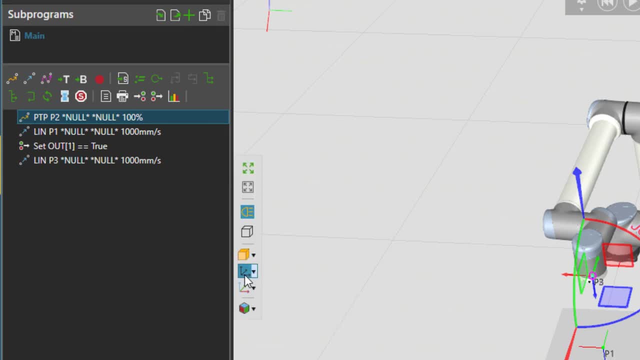 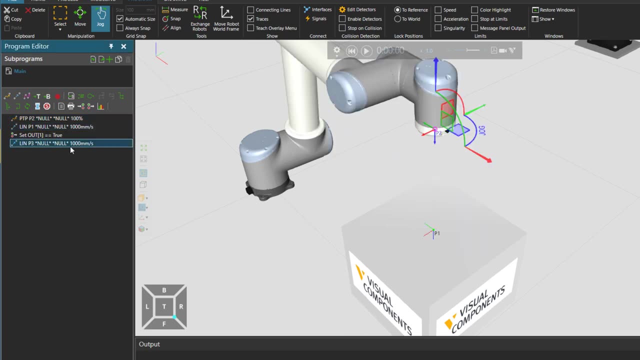 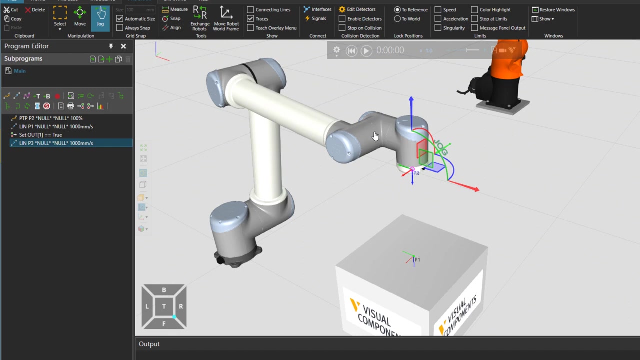 So right now, you see that I have in case that I can turn on these points. so you see that I have three points And when I choose one, the robot is going to that specific point with the joint values associated to it, based on the robot configuration for this point. 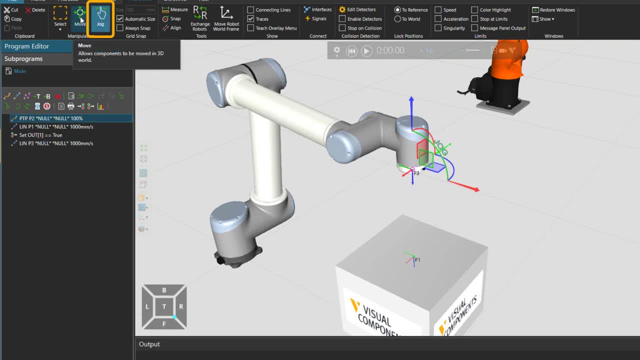 And the reason for this is that I am in the jog mode. So in case I choose the move mode, then you're able to choose the point without having the robot being jogged there. For example, this last point is P3.. I can move it over there. 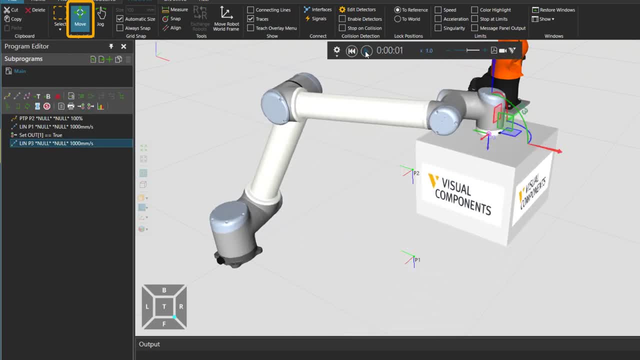 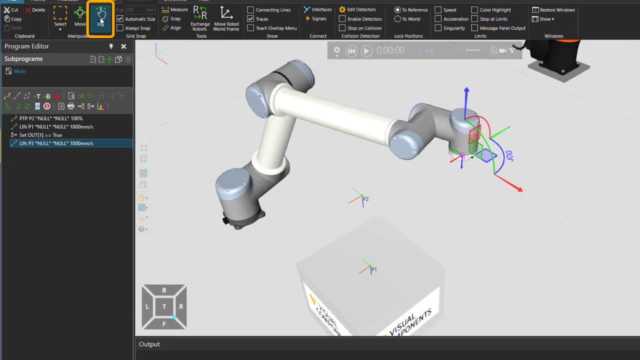 and then press reset, Robot picks the part and goes there And I'm still in move mode. But now notice, if I go to jog mode the robot goes to this new point. I can modify it when it's in the jog mode back and then just put it about where. 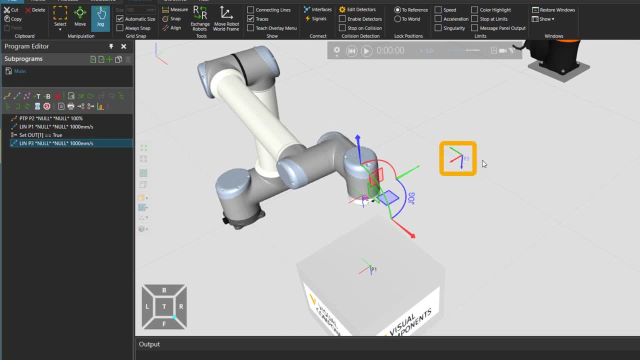 it was, But this is now not ready yet. If you want to change this P3 to this new location because we are in the jog mode, I need to use the touch up button. When I pressed it, you saw that this point jumped to where the robot end effector was And then reset, and 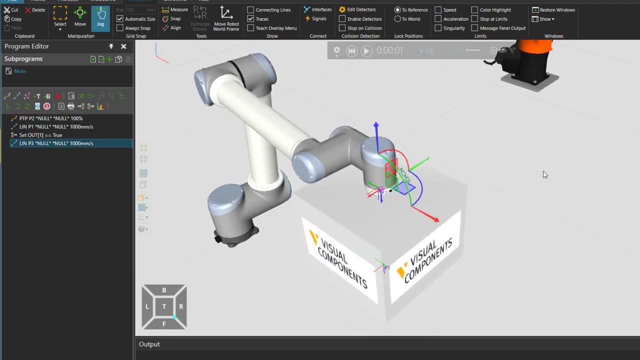 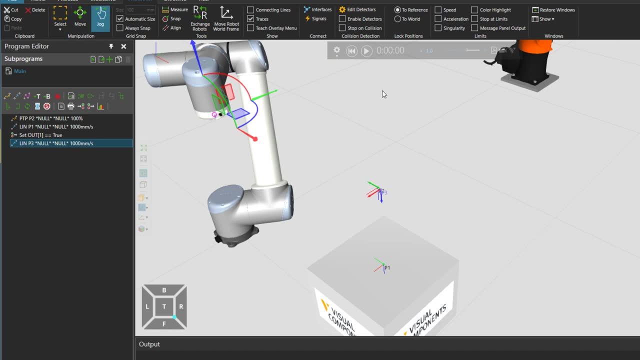 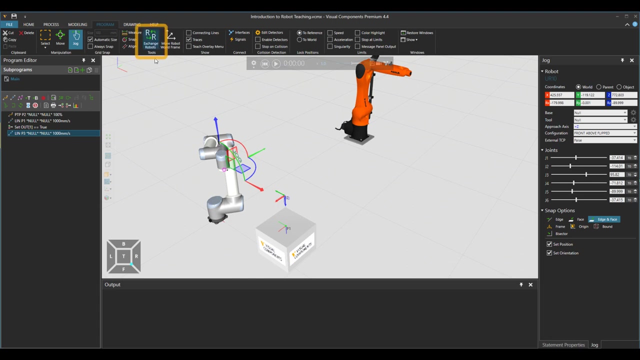 press play. So you see that it's using the new point To talk more about these tools up here. So we talked briefly about this manipulation And maybe one more that I would also talk about and implement it for you. here is the exchange robot. So let's say that you're not happy with this universal robot You want. 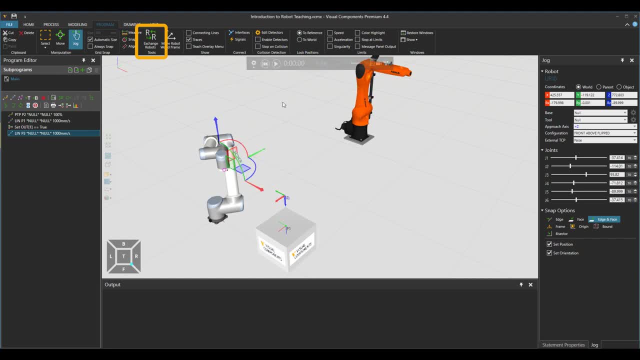 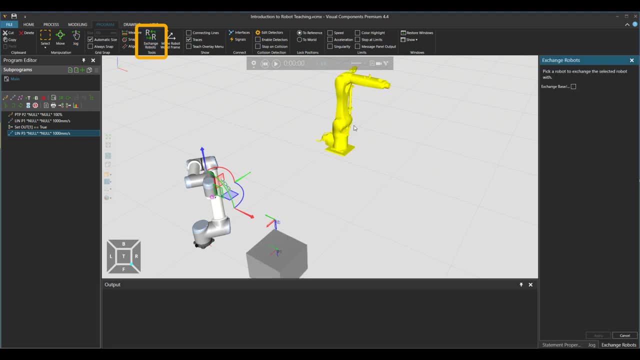 to change it, for example with this guy over here, the orange robot, And you don't want to do all the teaching again. That's okay, because we have the exchange robot button here. So let me just choose this robot, the new one, and then say that exchange all the. 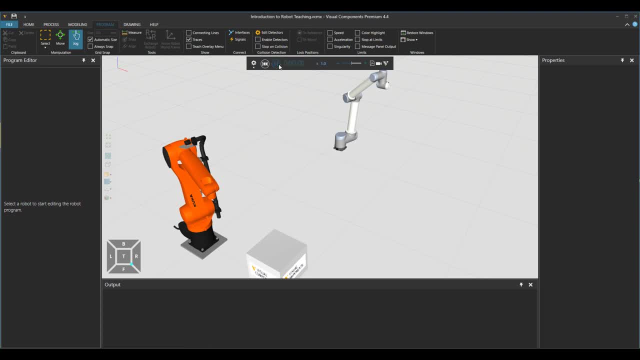 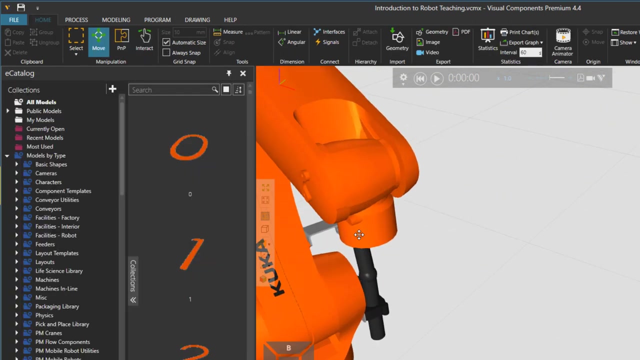 bases and everything and apply. So if I press reset, you see that my new robot goes and picks up the box. So it was as easy as that. Then let's go to have a tool, because the robot is just picking the box without any tool on it, And we have the robot tools in our E cat. 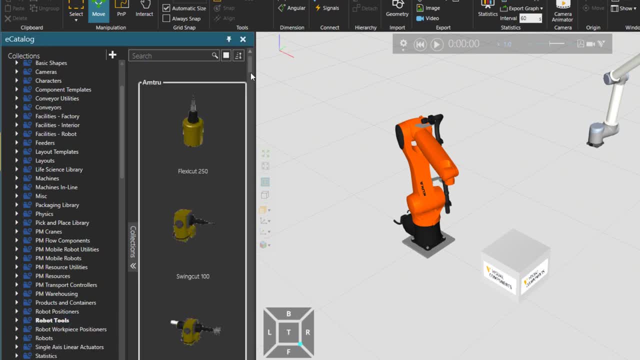 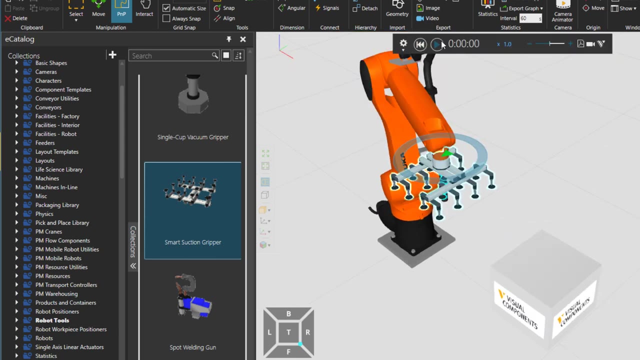 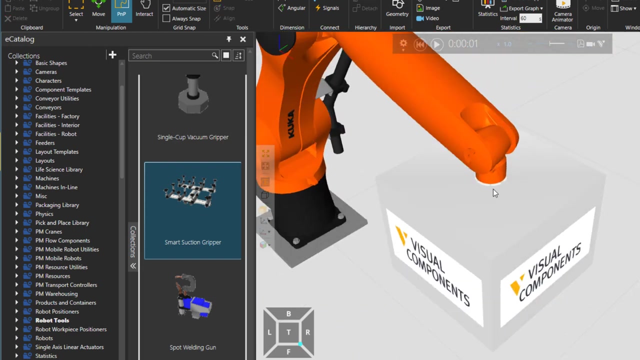 So I would scroll down and grab a tool. I would go to these tools at the end and maybe grab a suction gripper. so let's drag and drop it here and now I can just use that tool. oops, well, you see over here that now the tool is inside the box, and the reason 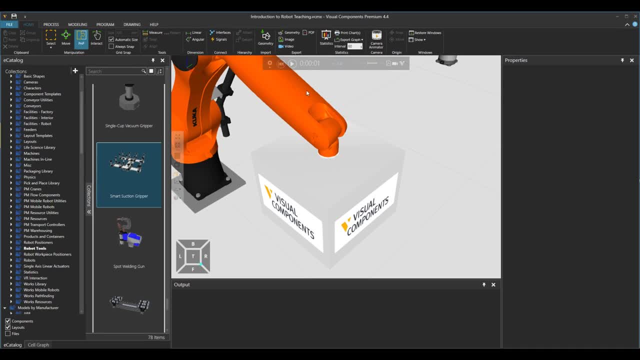 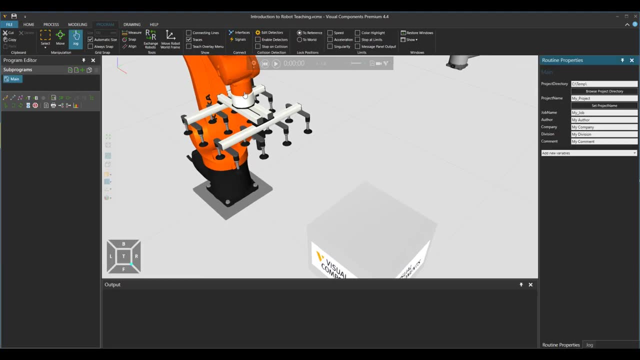 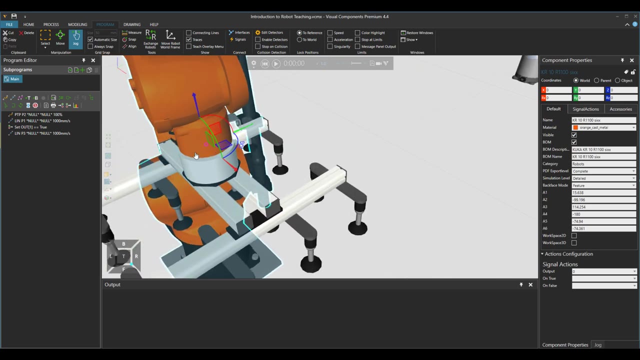 was that my tool center point, or TCP, is not set properly. so if we go back to program tab, you see that if I choose the robot and we are in the jog mode, the tool center point is now still on the robot flange. so we want it to be on the. 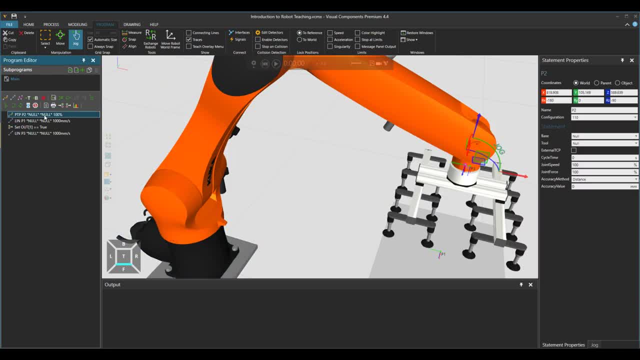 somewhere on the gripper properly. so I'm gonna just hold down control on my keyboard, choose all these points and when you look on the right side, these are the properties of each statement. so these statements over here they have. when you choose them, they have the properties on the right side. so I'm gonna choose here. 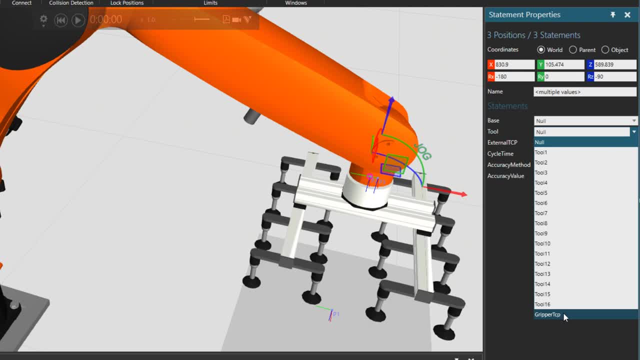 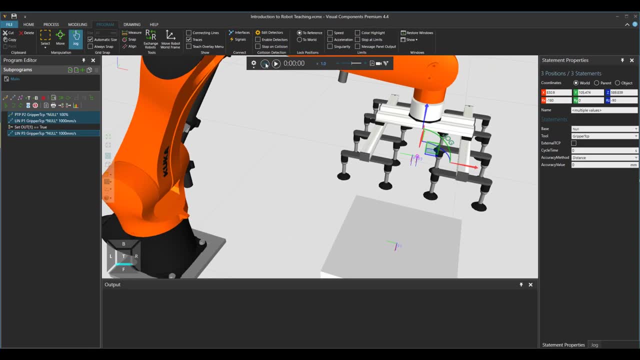 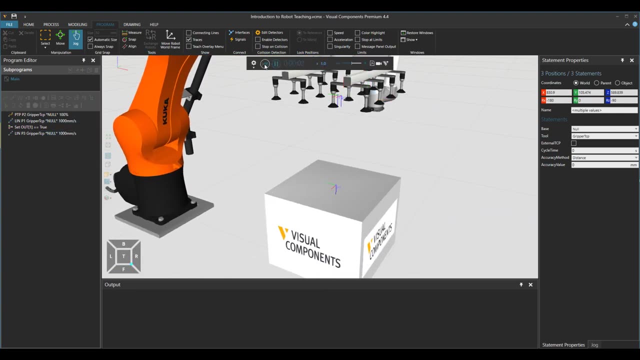 the tool for these points, and there is a gripper, TCP. this is a tool frame coming from the gripper, so right now that should work. so you see that. okay, so the robot did not go inside the box, but still it's not grabbing the box either, and I 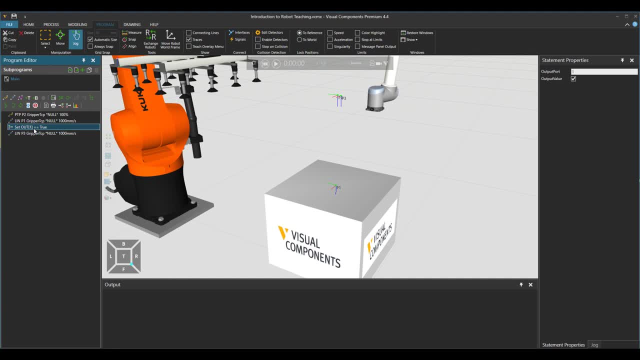 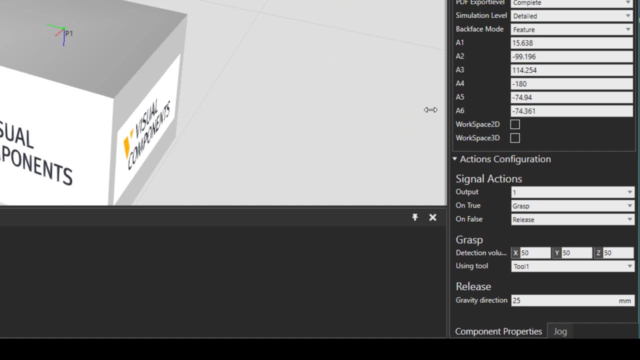 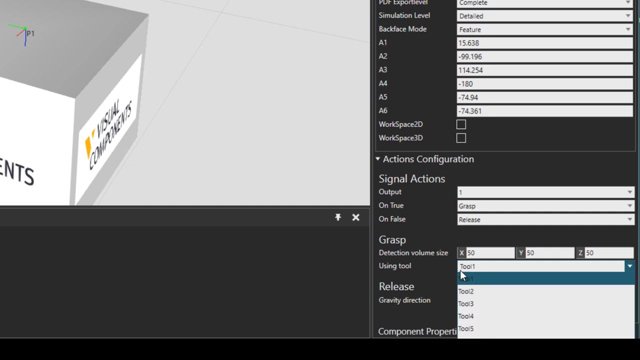 suspect that I need to check my signal that how it's working. so let me just click on the robot and go to action configuration in property panel, then go to signal one and you see over here let me just extend this menu. you see that grasping is using the tool number one, but I have to choose tool center point. 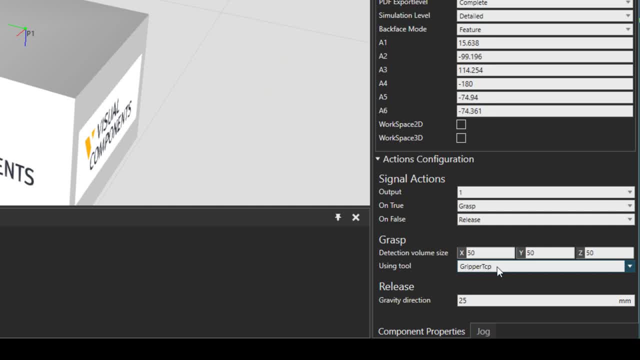 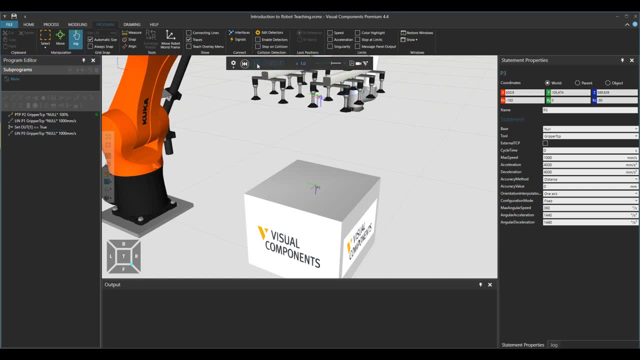 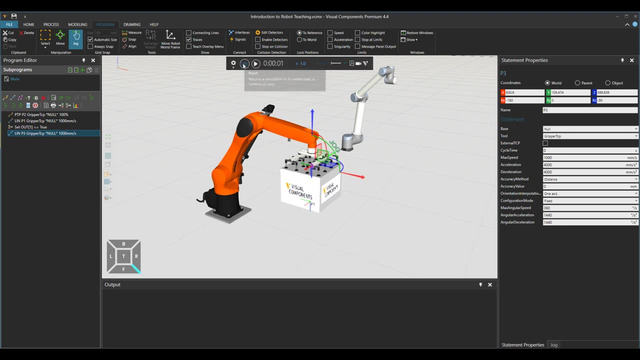 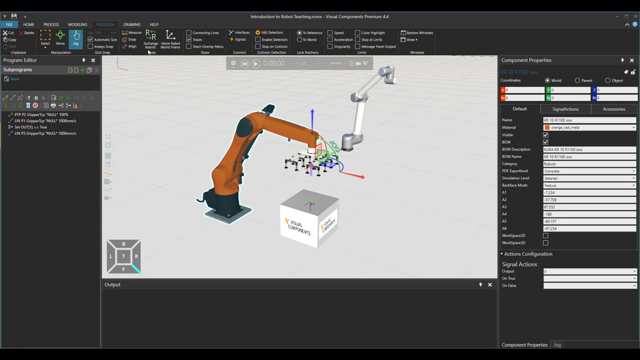 gripper TCP. so that is basically the right tool to use for these points, because these points are choosing gripper TCP. so if I press play, you see that robot goes and grabs the box. that's that you. so if I just go now click on this robot and say exchange with this, you are apply.